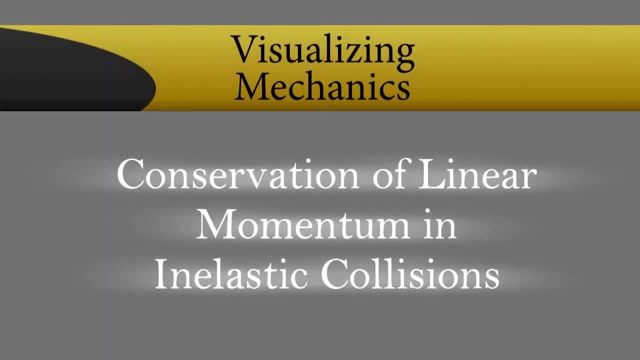 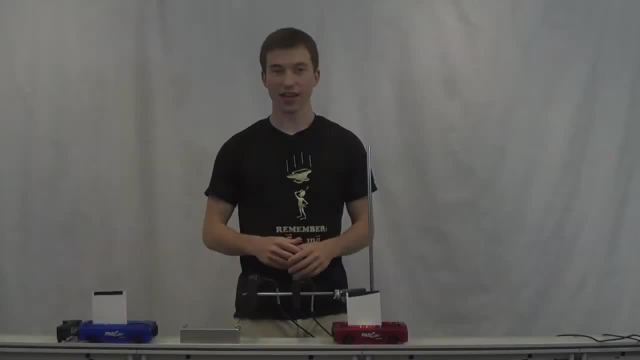 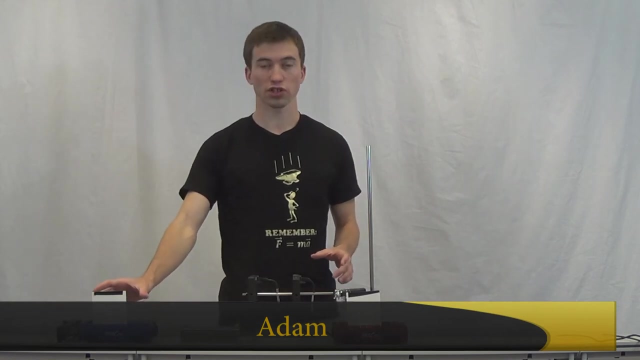 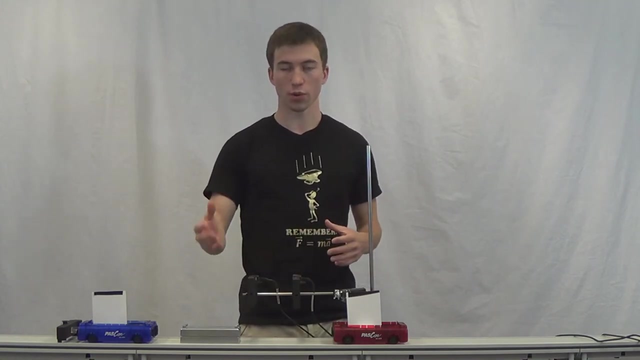 Today we're going to be examining inelastic collisions using these dynamics carts and these masses. By having this cart start with an initial velocity and colliding it with a stationary cart, we're going to see how velocity scales when you add additional mass to the system. We're going to use Velcro to model an inelastic collision and we're 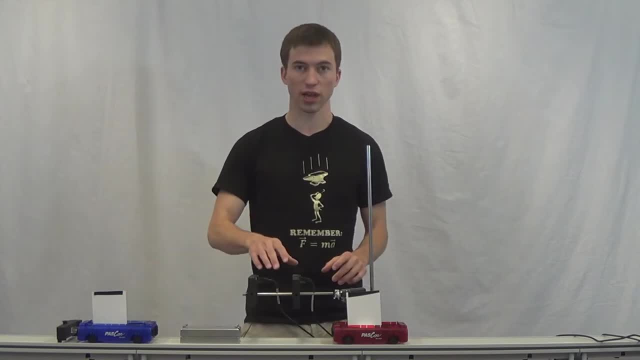 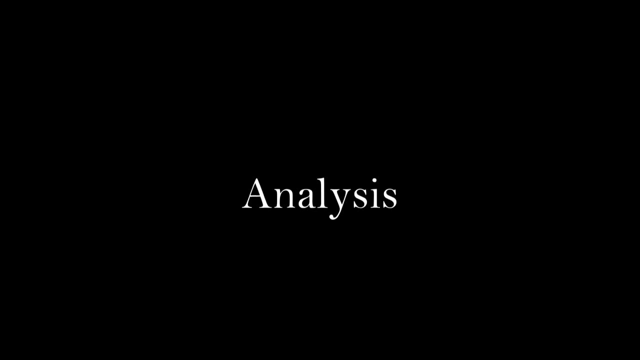 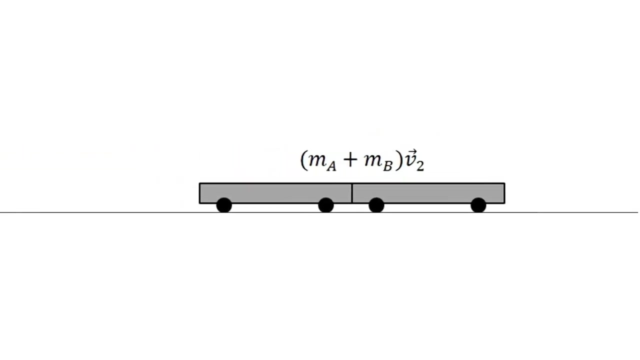 going to compare our initial velocity using these photogates with our post-collision velocity using the same setup. In this experiment, we will be examining the conservation of momentum of an inelastic collision and the energy loss as a result of that collision. To understand, 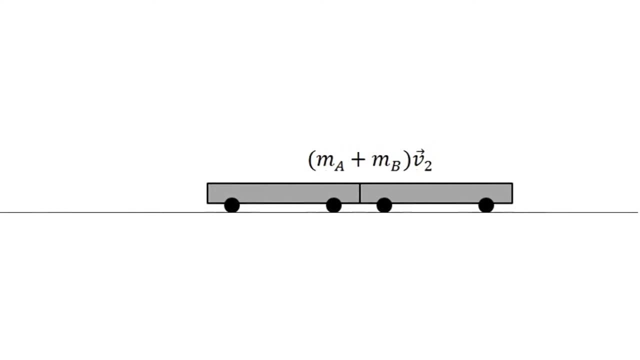 the collision we will break our system into two times: one pre-impact and two post-impact. Prior to impact, our momentum is given to us entirely by cart A as it begins with an initial velocity here- VA1, while cart B begins at rest. When we look at our system- post-impact- 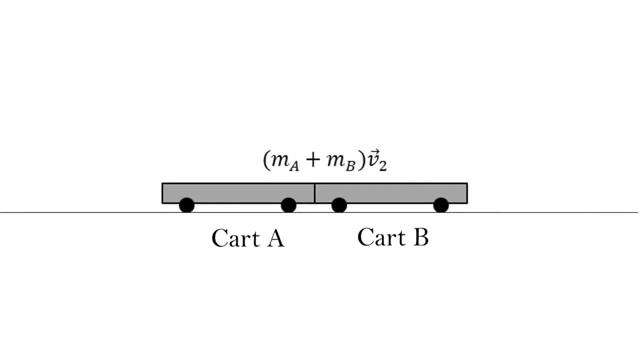 we now have to account for the masses of both cart A and cart B, Because they collide. in an inelastic collision. they will have the same velocity, V2.. Knowing this and working from our conservation of momentum, we're going to see how velocity scales with an inelastic 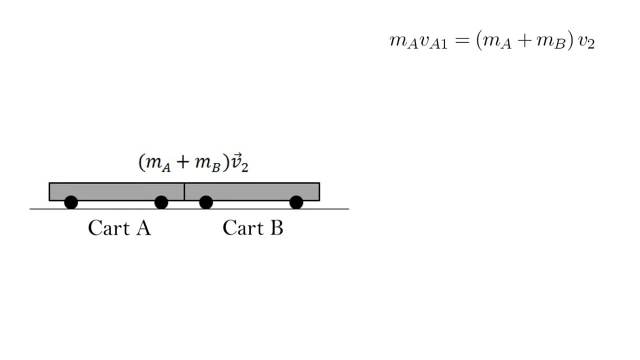 collision. To compute the ratio of the final velocity to the initial velocity. we can solve for the final velocity- V2, in terms of our masses and our initial velocity, which we will measure. Also, we can compute the ratio of the final velocity to the initial velocity in terms 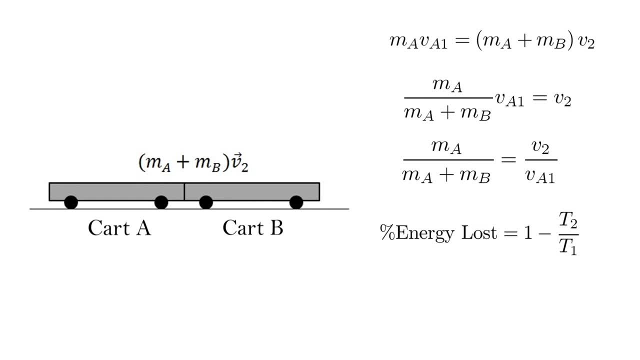 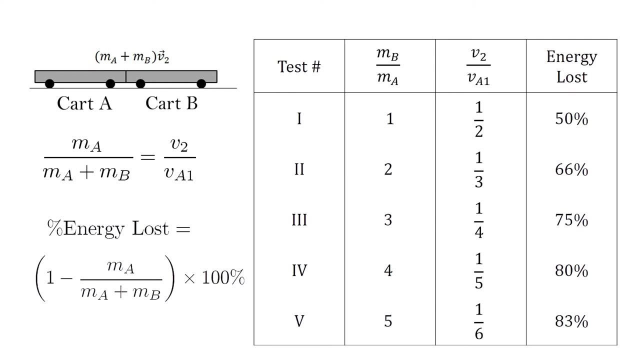 of the masses alone. Using kinetic energy, we can also calculate the percent energy loss of the collision in terms of simply the mass. We break this experiment down into five cases. We take each process to a test with a varying mass of V, ranging from equal to the mass. 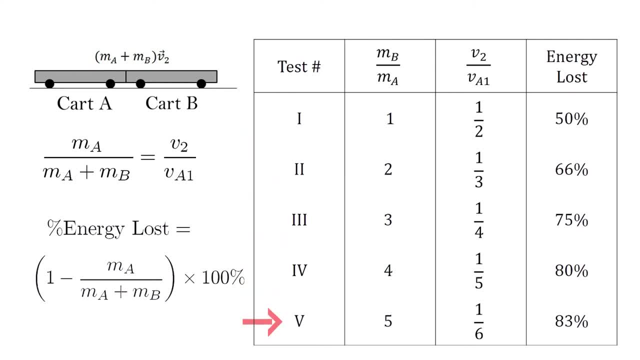 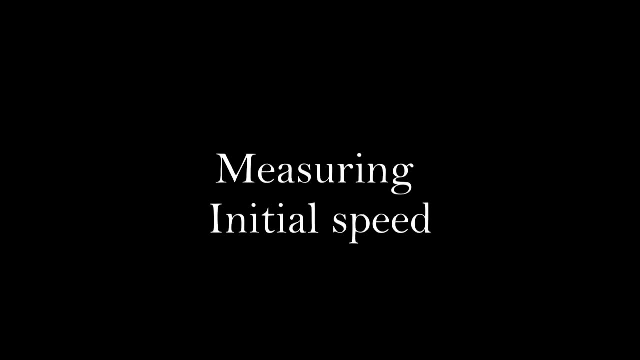 of cart A to five times the mass of cart A. We will predict the velocity on the system post-collision and compare it with the velocity prior to impact. We will also calculate the percent energy loss for each case. To begin our experiment, we will first measure the initial velocity of the cart: 0.76 meters.